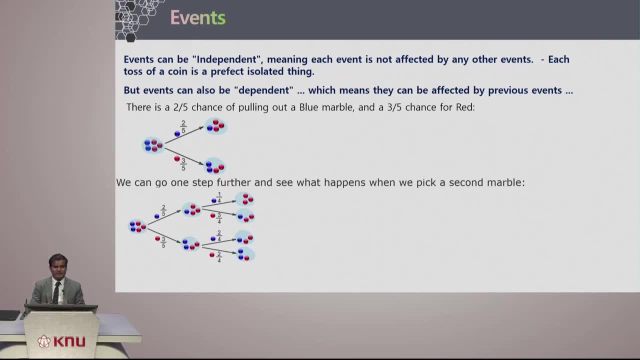 we already discussed about what is conditional probability and what is conditional probability, What is an independent event and what is an dependent event. Well, we know that when you toss two coins, those coins are kind of independent because none of the previous experiments is 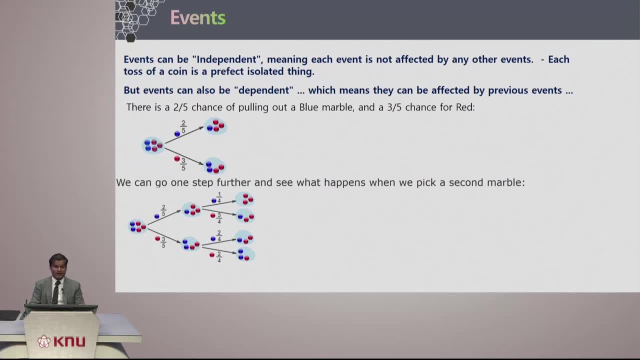 going to affect the current one, So event can be independent, meaning each event is not affected by any other events, Just like tossing a coin is. each time you toss a coin is perfectly an isolated event. it is not influenced by the previous toss or the toss. 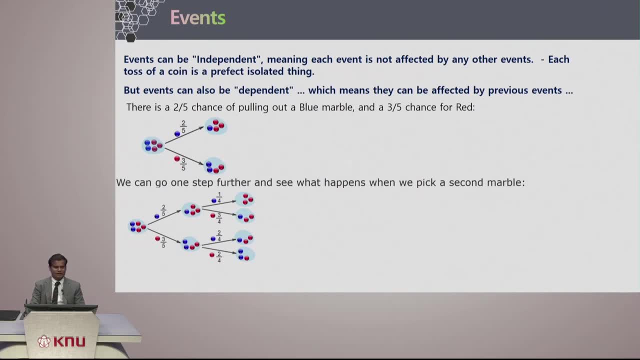 to come, But events can also be a dependent, which means they can be affected by previous events. Consider this example here. So you can see there are five marbles in this bag and three red marbles and two blue marbles. So there 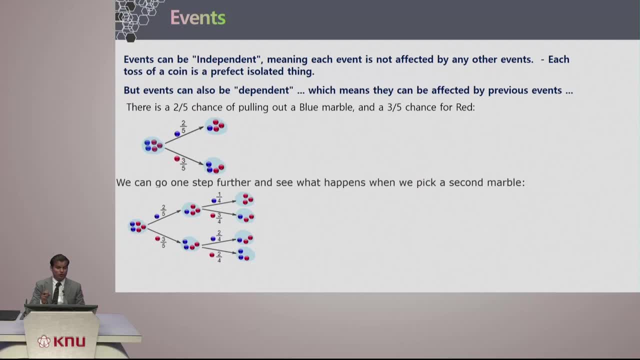 are two by five chance of pulling out a blue marble and three by five chance for a red marble. Just go one step ahead and see. See what happens when we pick the second marble. You can clearly see that in the first step. for example, if you pick up this blue marble, 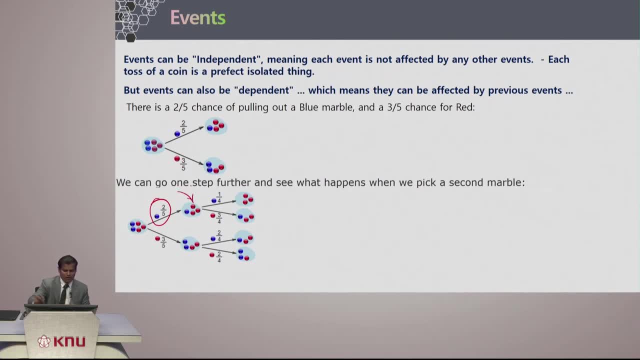 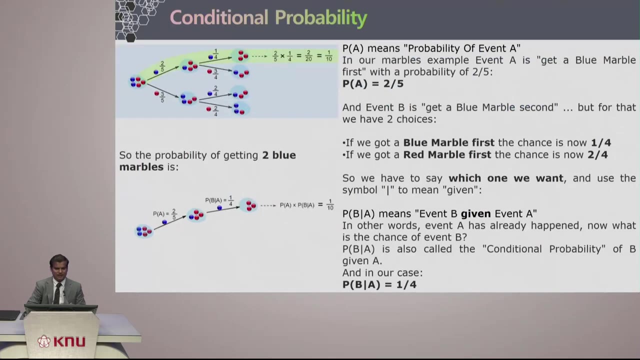 then your probability might change drastically in the next step, because right now there is only four marbles And now your probability of picking up the blue marble changes. So that is what is being illustrated here. So we can consider these events as individual events, Though they are individual events. 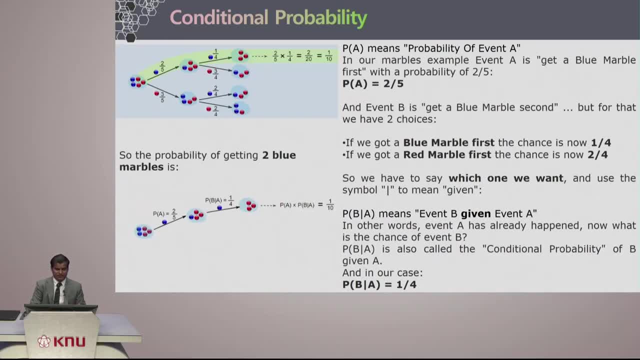 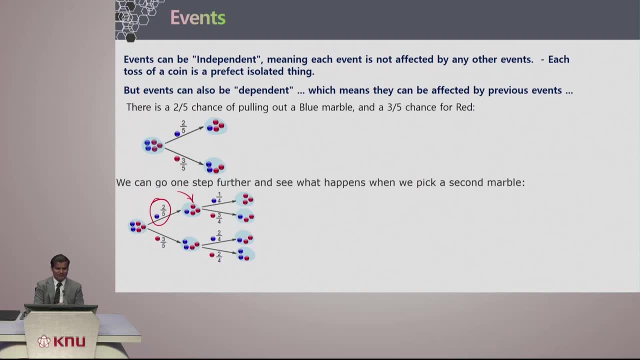 still. they each depends on the previous events, Just like here. you see that if you already picked up a blue marble and second time when you pick up the blue marble, the probability changes to one by four. Likewise, if you pick up the red marble in the first instance and 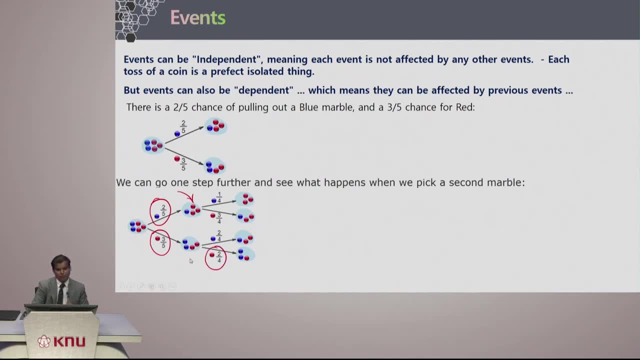 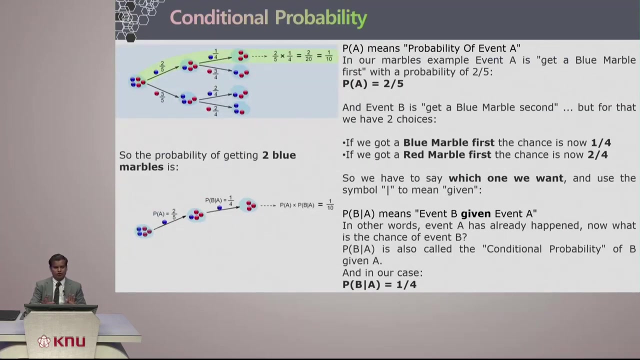 for the second instance, picking up the red marble, the probability changes to two by four, So on and so forth, Because of the previous events. Yes, now you can see that how these events are depend on one another. With this basis, let us deal more on how this conditional probability works, As the word condition applies. 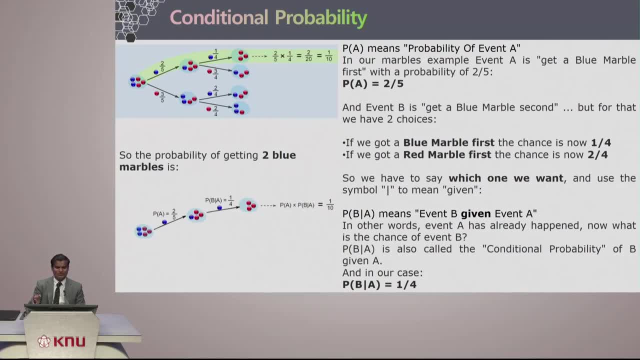 and implies we know that it has to satisfy certain conditions, Just like when we say P of A, which means probability of event A. in this example of our marble, the event A is get a blue marble first, with the probability of 2 by 5.. The same thing that we have seen. 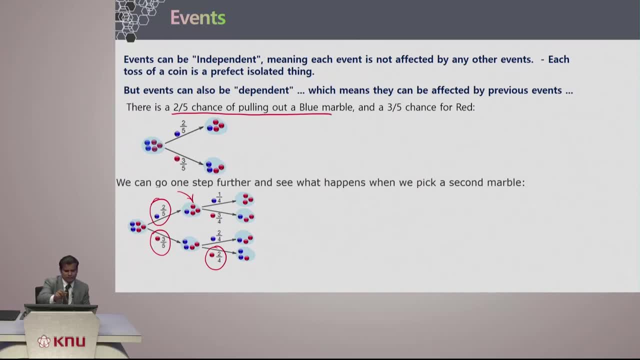 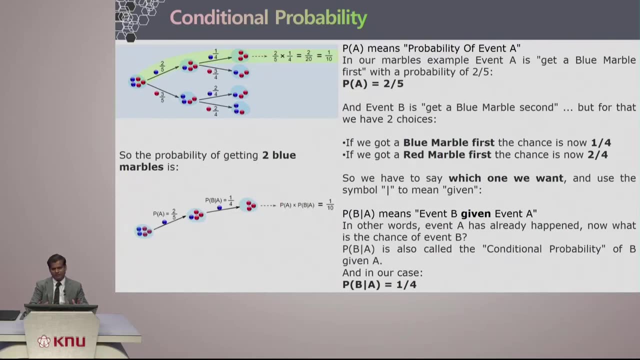 here For getting blue marble. it is 2 by 5.. Yes, let us consider that as the event A, So P of A is 2 by 5 and event B is 2 by 5.. Get a blue marble second. but for that we have two choices. If we got blue marble first, 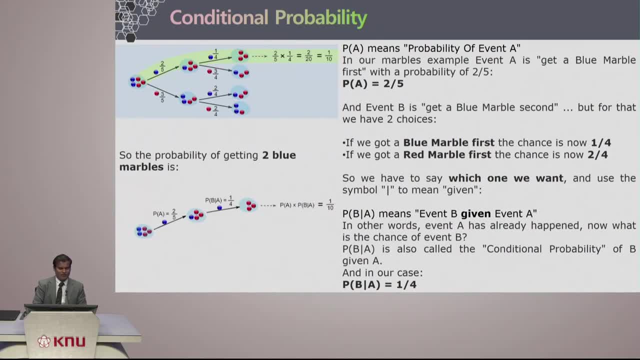 the chance is 1 by 4. and if we got red marble first, the chance is 2 by 4.. You got it If you got in the first time. if you got blue marble, then your chances becomes 1 by 4. the 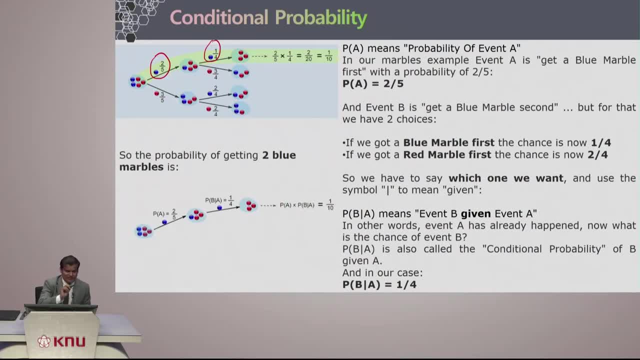 second time, But in the first instance, if you get a red marble, your chances become 2 by 4 for picking up the blue marble in your second chance. So we have to say which one we want and use. we can use the symbol just like a bar. 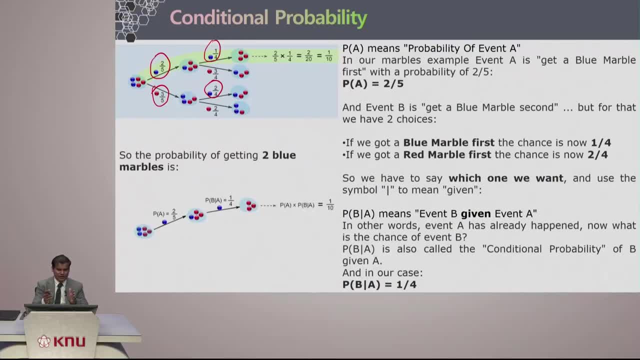 which means given. So you can look closely here: Probability of B given by B. So P given A. That is what it says. P probability of event B is given, event B given event A, which means that we have event A which is already given to us and we have to estimate. 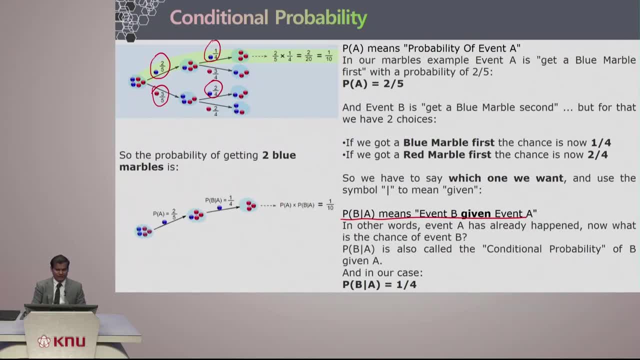 for event B. So event A has already happened and now you want to estimate what are the chances for event B. That is what this means: probability of B given A. So this probability of B given is called the conditional probability of B given A. So in this example we can: 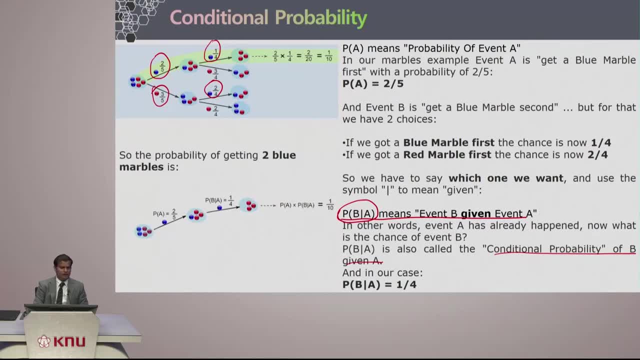 see that probability of B given A is 1 by 4. In this case when we have the blue marble picked up In the first instance. So let us try to build up So you can see here step by step. you. 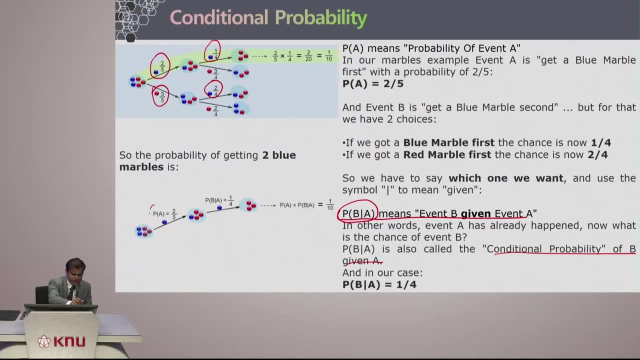 can see what is happening. Probability of A initial probability right Probability of A is nothing but get a blue marble first. In the first chance you are getting the blue marble And probability of getting the blue marble again in your second chance is 1 by 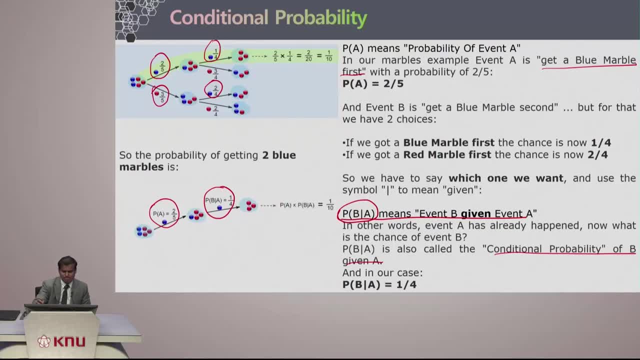 4. That is probability of B given A. So probability of E given B. we want to check that out. So this is the basis for the conditional probability. We know that, given a condition, what is the probability of B given A? We know. 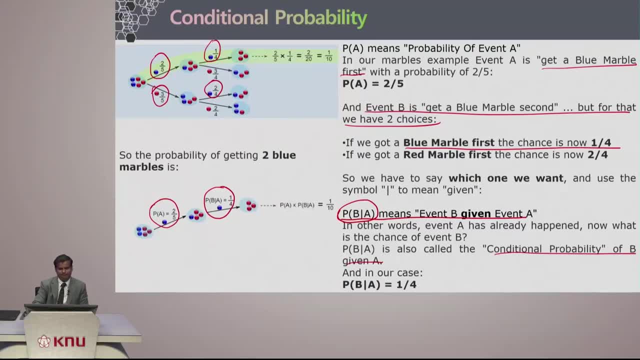 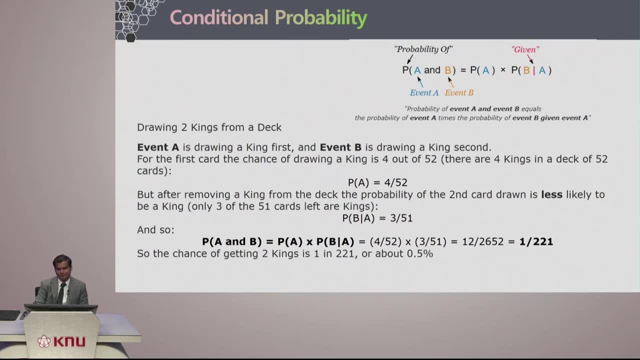 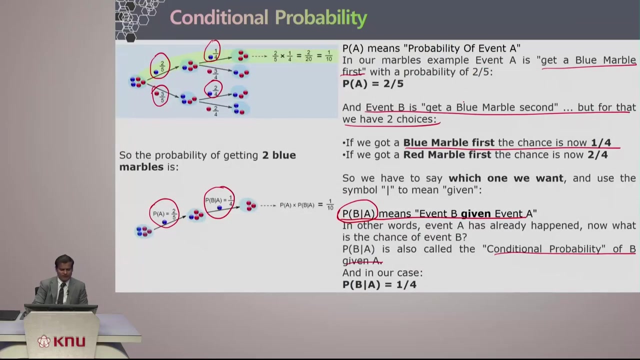 is the chances for another event. So with this thought we can define: what is this? conditional probability is So probability of A and probability of B, or event A and event B. we can say probability of A times probability of B given A. So just like here, probability of A times probability. 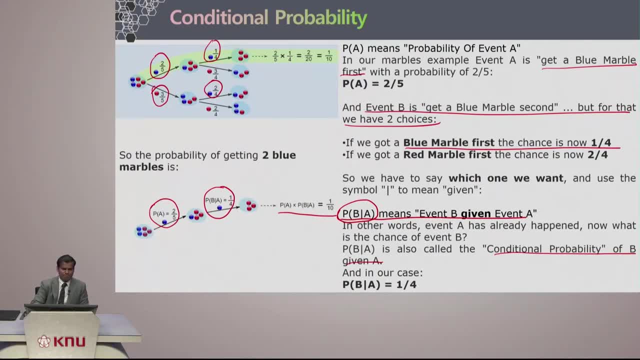 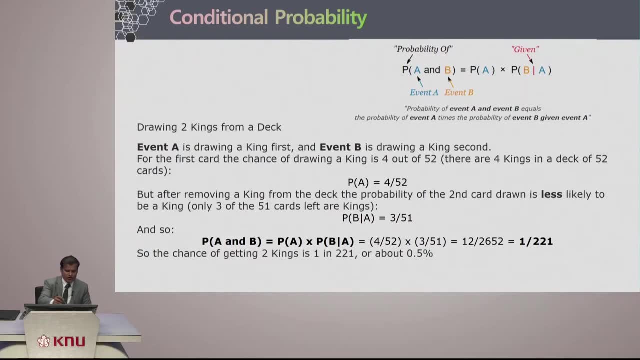 of B given A. So in this, with this thought, let us move on to some simple examples of drawing two kings from a deck. You have a playing cards and you want to draw two kings. Event A is drawing the king first, the first chance, and event B is drawing a king in your 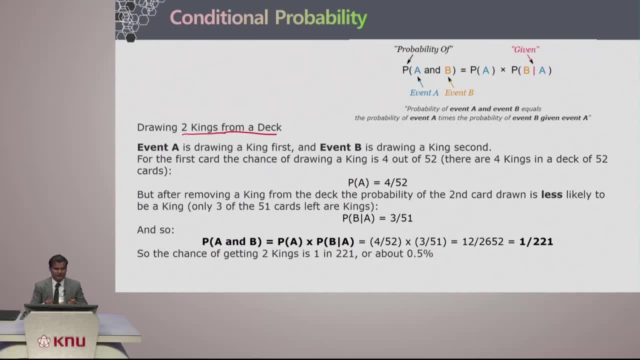 second chance. So for the first card, the chances of a king is 4 out of 52, right? So that is your first option. probability of A is 4 by 52, since you know that 4 kings are in your deck of 52 cards. But after removing 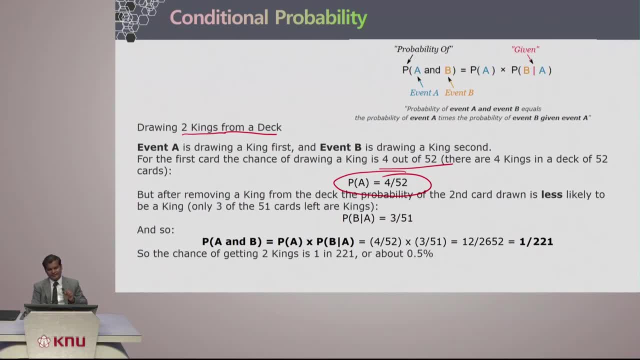 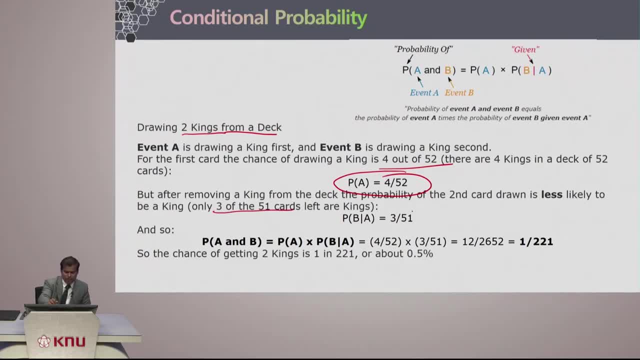 3 out of 52.. 3 out of 52.. 51 cards are there. So that is probability of B, given that probability of A has already happened. probability of B, given A. probability of B, given that the event A has happened. 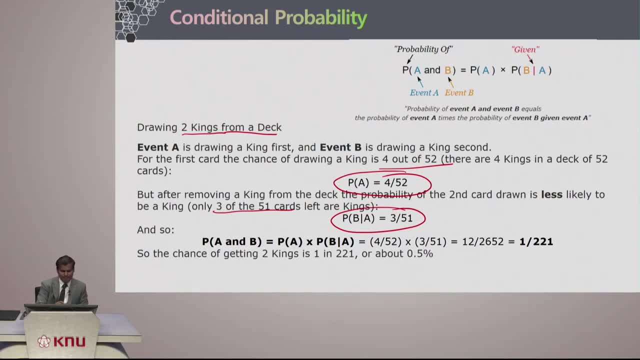 So we could write it this way: probability of A and B, So we can say probability of A times probability of B given A. So when you multiply that you get 1 by 122.. So it is about around like very less probability there, around 0.5 percentage. So that is. 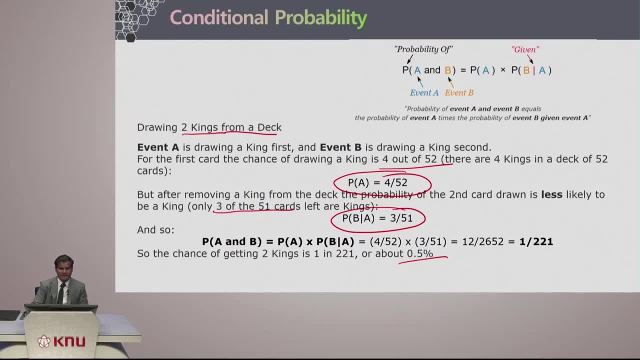 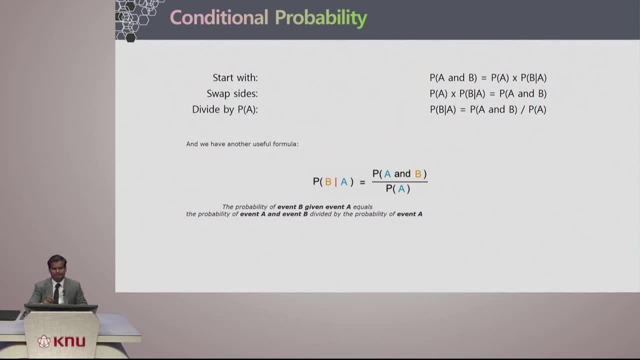 an example. Let us, with this example, let us move on and see How things can be worked out. So initially, you start with probability of A times probability of B given A and you can swap this around and you can also divide this by probability. 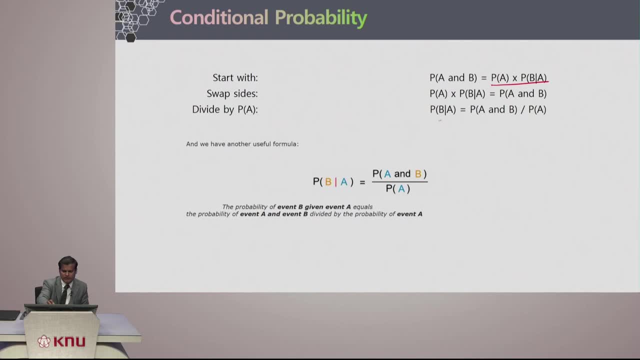 of A. So when you divide by probability of A, you come up with this form. In other words, we can use this formula. This is quite useful formula there. probability of B, given A equals probability of A, and B divide by probability of A, Or in other words, the probability of. 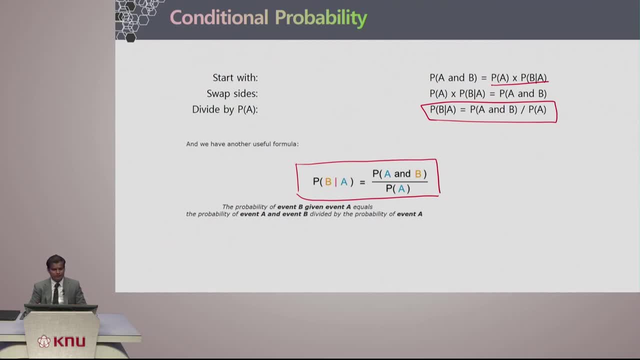 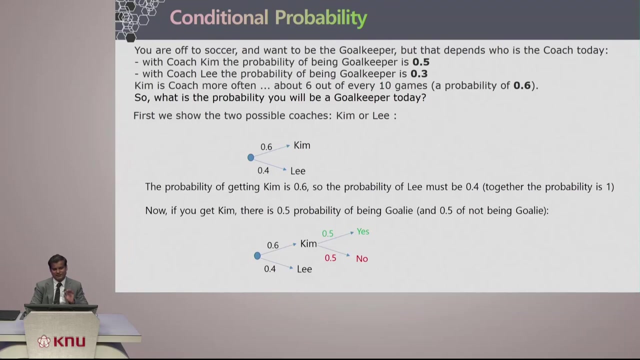 event B, given event A is equal to probability of event A and event B divide by the probability of event A. So here is another real time example. So it is about probability of A example. You can look at this example closely. So you are off to soccer and want to be a. 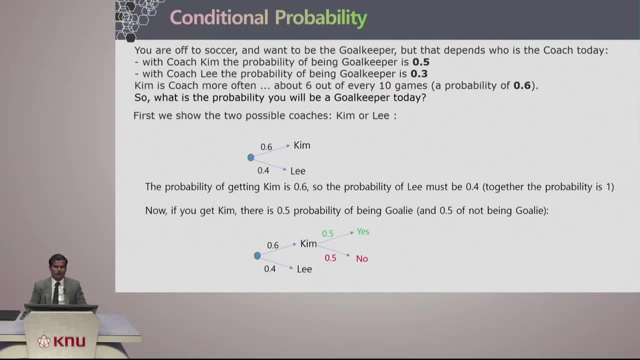 goalkeeper, but that depends on who the coach. today, With coach Kim, the probability of being goalkeeper is 0.5 and with coach Lee, the probability of being goalkeeper is 0.3.. Kim is coach more often and about 6 out of every 10 games. that is probability of 0.6.. 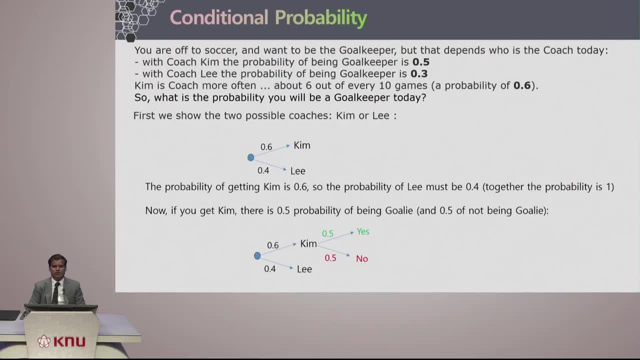 So what is the probability that you will be a goalkeeper today? Well, let us see the two possibilities. like we right away know that probability of Kim being the coach is 0.6 and probability of Lee should be 0.4.. And if you get Kim, there is 50 percent or 0.5 probability of being a goalie. right? 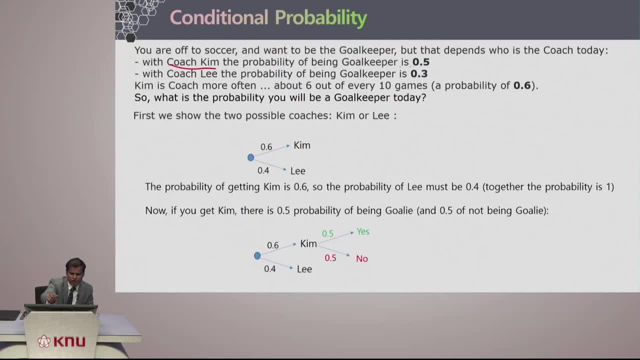 If Kim is the coach, you have 0.5 percent or not 0.5 percent. it is 0.5 probability of being a goalie, And if it is Lee, then it is going to be 0.3.. 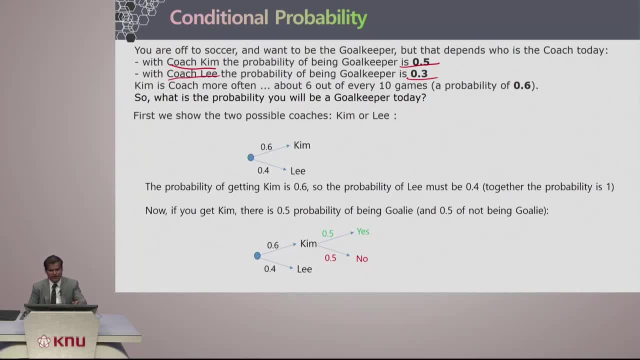 So we can put that in this tree graph. You can see you have a chance of 0.5 being a goalie. if Kim is the coach, Then for Lee, if he is the coach, then you have 0.3 probability. 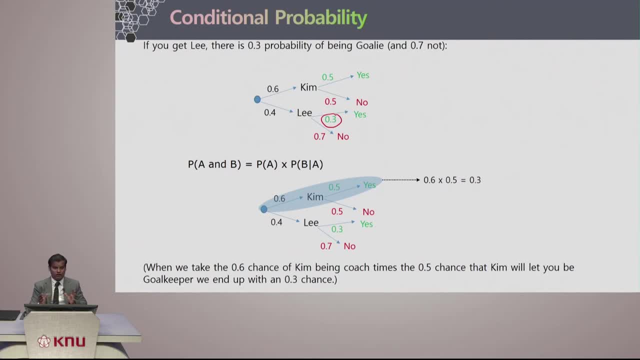 So we are putting out all the possible probabilities and we are trying to figure out what happens if probability of A and B equals probability of A times. probability of B equals 0.6.. So let us think about this. So if Kim is the coach and it is 0.5, then it is 0.3.. Let us 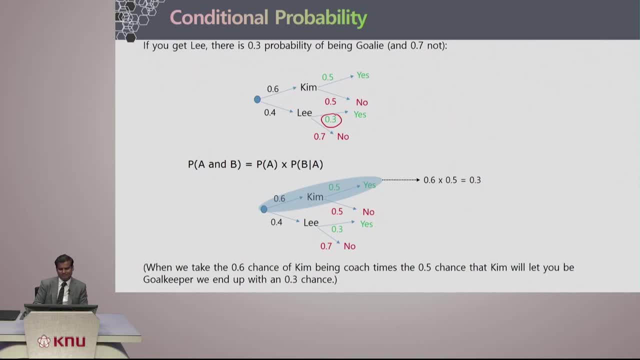 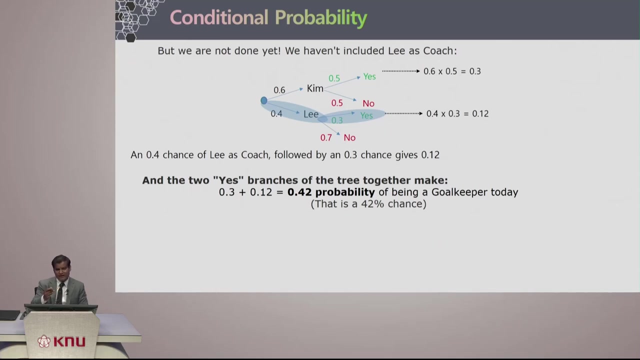 A times probability of B given A. So when you take this 0.6 chance for Kim being a coach, which gives 0.5 chance that Kim will let you be a goalkeeper, and we end up with this 0.6 times 0.5, which is 0.3.. But you can clearly see how it happens. what if Lee is the coach? 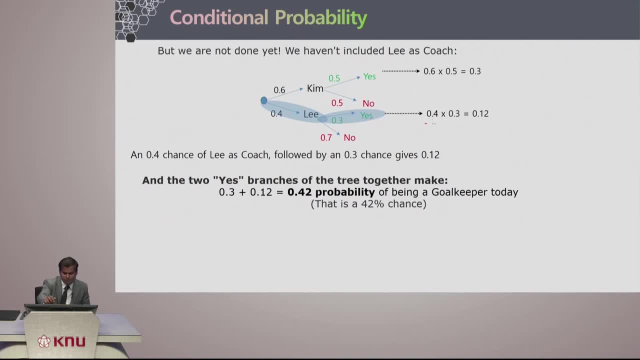 The same thing applies here: 0.4 times 0.3, which is 0.12.. So we have this: branches out of this tree which says yes and no: Yes, you can be a goalkeeper and no, you cannot be a goalkeeper. So when you add up these, 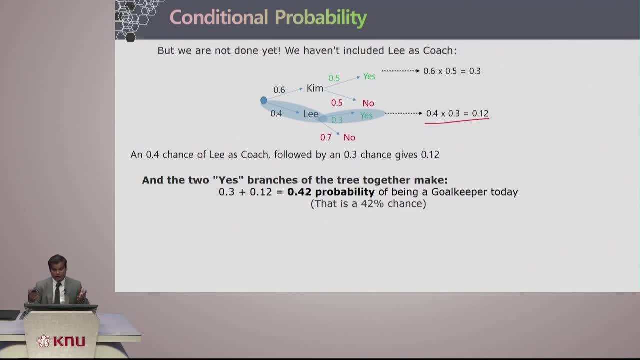 chances. with the probability of Kim and Lee, you get 0.3 plus 0.12, which is 0.42 probability of being a goalkeeper today. In other words, you have 42 percentage chance of being a goalkeeper. So can you see that how one event is affecting another event? 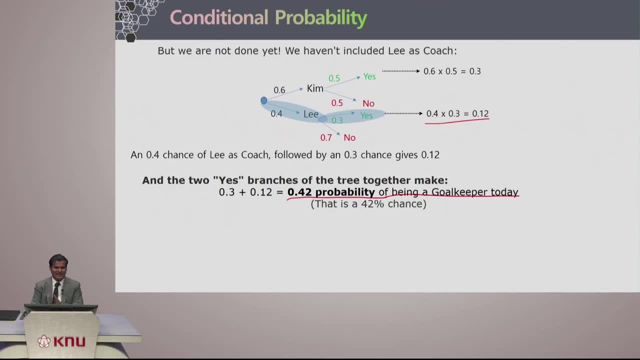 You are talking about the goalkeeper. You are talking about the goalkeeper. You are talking about you being a goalkeeper, but that really depends on other factors. So that is how we are building up, So you can see the overall probability of even not being. 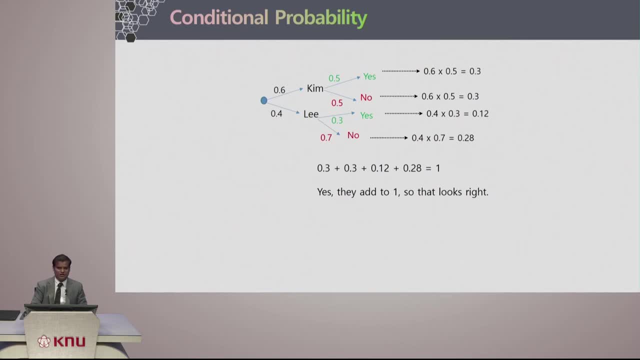 a goalkeeper. So you can see how this going to be add up. We know 42 percentage. you cannot be a goalkeeper, or you can be a goalkeeper, which means 58 percent chance you are not. It is like 0.58. That is you do not get a chance. but anyway, if you add all those stuff, 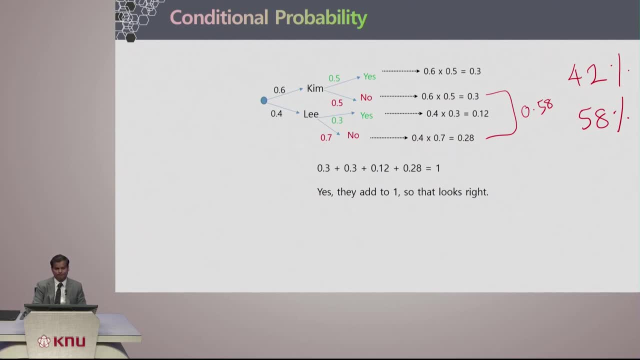 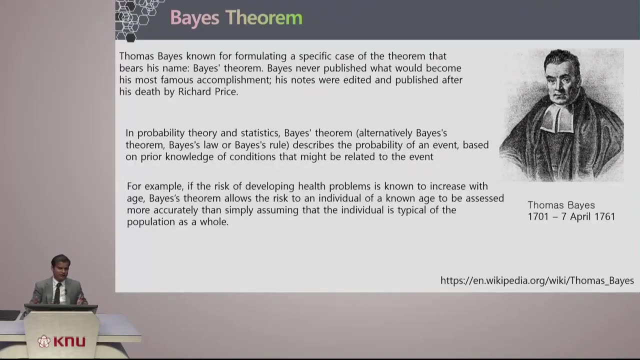 you can get 1, the overall probability. Let us move on to this Bayes theorem. As we have seen what is the conditional probability and now Bayes theorems are based on this conditional probability and we can see how this is going to help us to formulate various cases. So 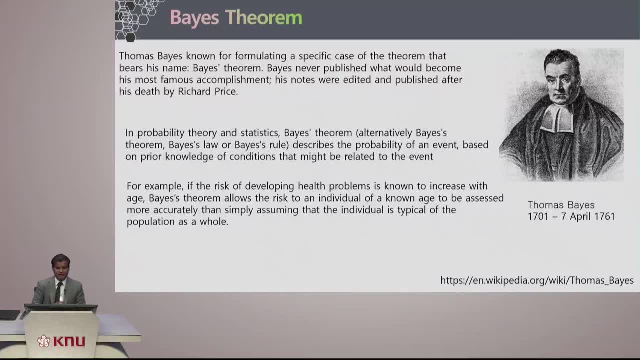 this has been formulated by Thomas Bayes, and he is in fact contributed a lot to this statistics by means of his Bayes law and Bayes rules, Though he did not publish his original work. this work, in fact, was published by Richard Price after Bayes death. 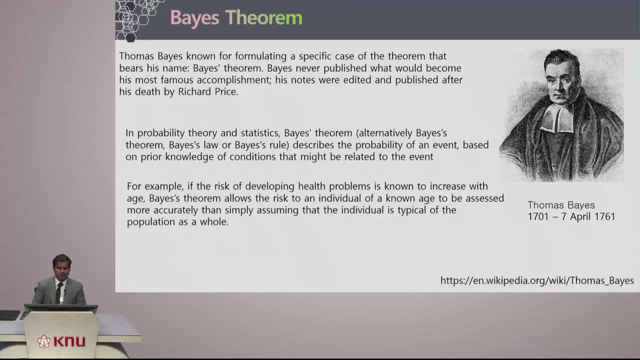 So basically, this is how the Bayes theorem goes on. Here is an example given to us. like if the risk of developing health problem is known to increase with age, then Bayes theorem allows the risk to an individual of knowing age to be accessed more accurately than simply. 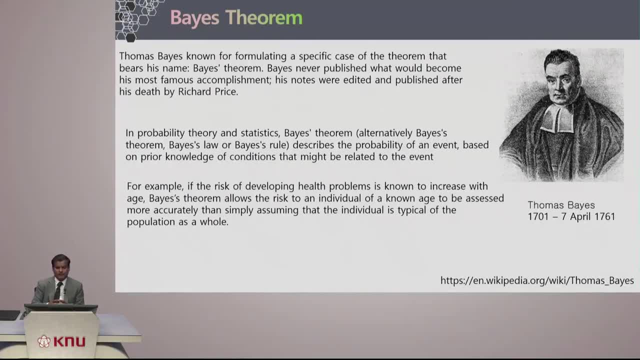 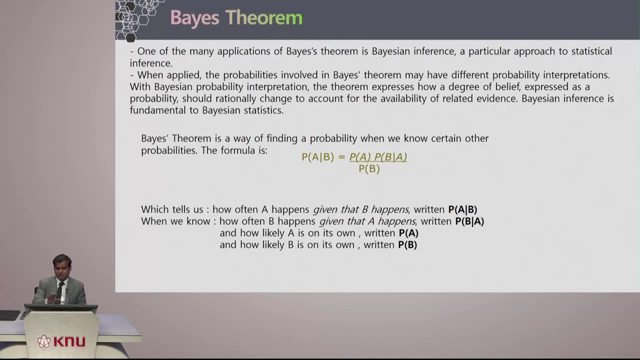 assuming the individual is typical of population as a whole, So he is considering other factors that would affect this particular event. So, to be precise, we could say that the risk of developing health problem is known to be greater than the risk of developing age. 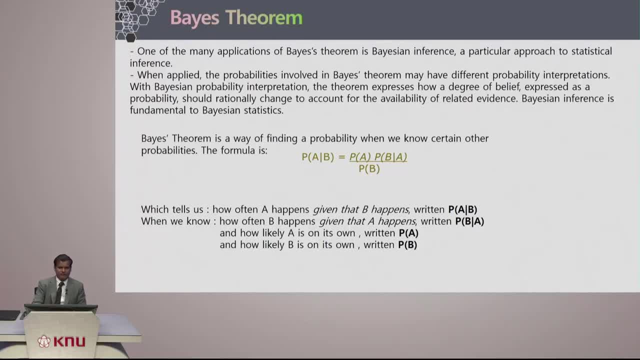 So the Bayes theorem is also very similar to what we have seen, that is, the conditional probability. Yes, when we say Bayes theorem, as you can see, it is applied in various Bayesian interference. So Bayesian probability interpretations can be expressed in various things, Even they. 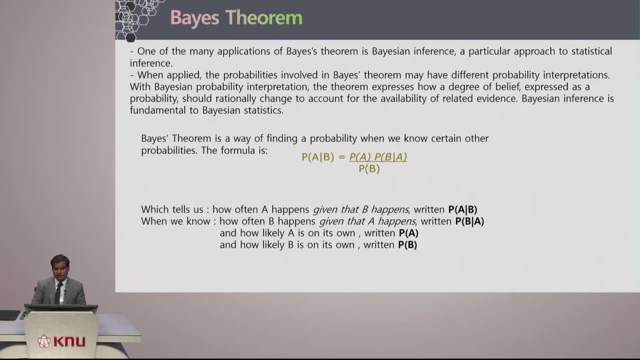 have something called Bayes networks, Bayesian networks and belief networks. they are also being formulated And this Bayes statistic is one of the basis for that. So if you want to find probability based on this Bayes theorem, you can see probability of A given B. probability of A given B equals. 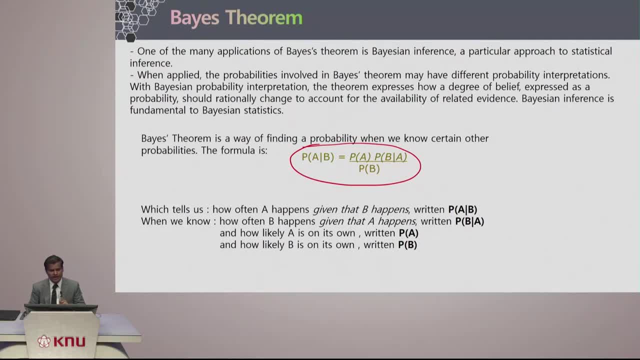 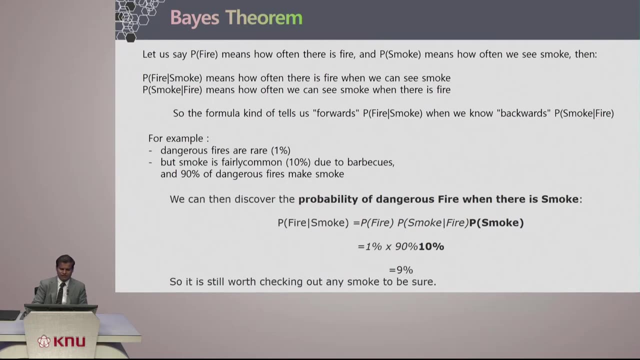 probability of A times probability of B, given A divided by probability of B. So with this basis we will move ahead and discuss more on this. Here is one example. Let us say probability of fire means how often there is a fire and probability of smoke means how often we see smoke. So probability of fire given smoke. 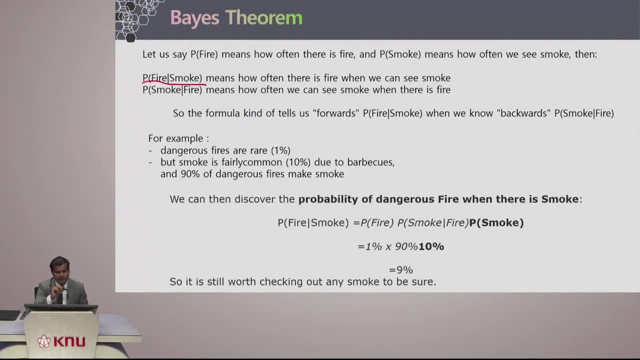 which means that how often there is fire when we see smoke, And probability of smoke given fire means how often we see smoke when there is a fire. So, based on that, let us formulate this whole thing with forward probability of fire given smoke and for backwards probability of smoke given fire. And there are some information. 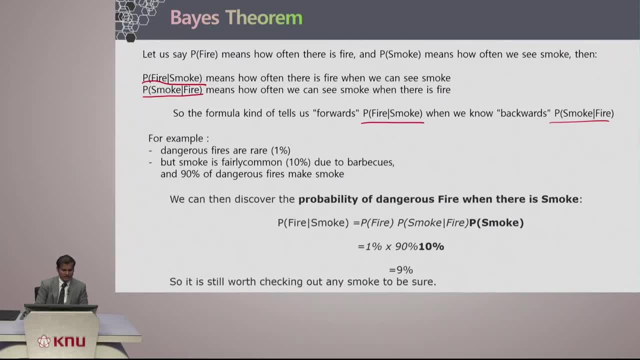 given to us while solving this problem. like the dangerous fires are rare, which means like 1 percent chance of getting a dangerous fire, But smoke is fairly common- like 10 percentage- because many people might do barbecues and things like that. 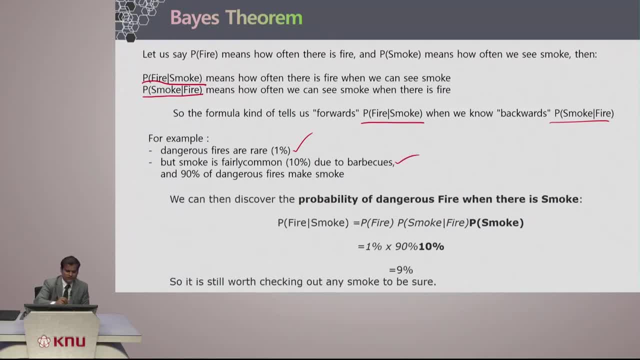 So smoke is quite common. 90 percentage of chances, or 90 percentage of dangerous fires make smoke. Whenever there is a dangerous fire, 90 percent, we see smoke. This is the third factor. So with these factors, let us see what is the probability that we have. 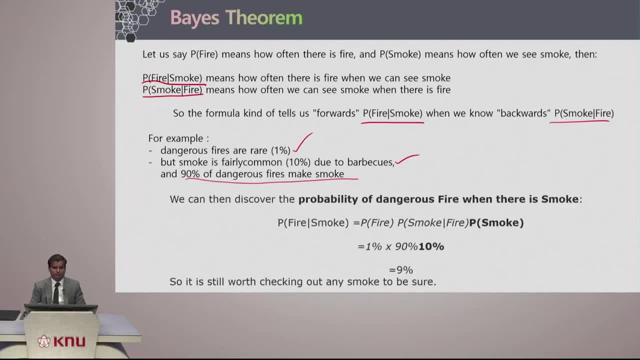 here for smoke. So we can see here the probability of fire is rare, very rare even, which is 1 percentage And probability of smoke, given there is a fire. So whenever there is a fire, there is 90 percent chance that you have a smoke. So we are going to have this. 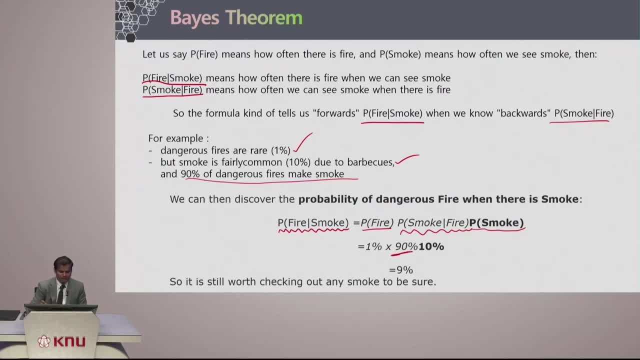 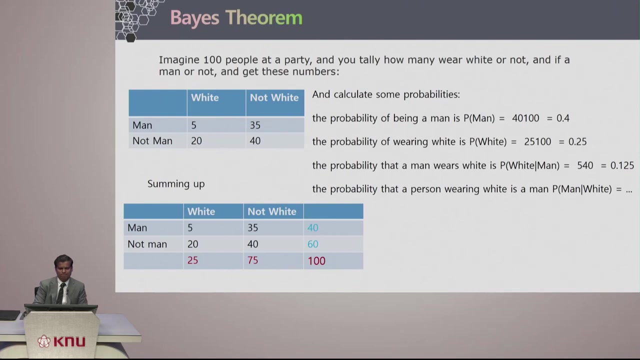 90 percent given to us here. So eventually you can find that it is around 9 percent chance that we have. So with this thought we can see how we can apply this conditional probability to Bayes theorem So we can expand more on this Bayes theorem. We can consider imagine: 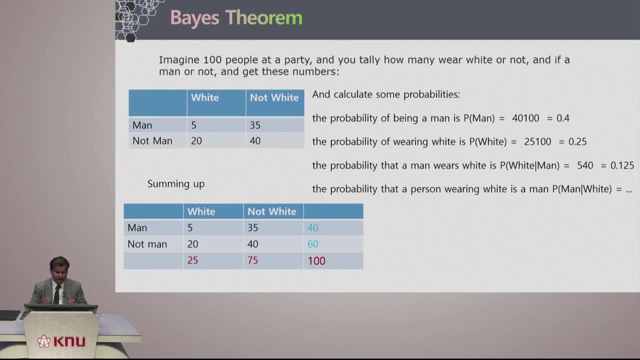 that 100 people are at a party and you want to know, or you want to tally, how many people wear white and how many people do not wear white, And if a man or not a man. when you have guest in the party, you want to consider whether he is a man or not. So probability- 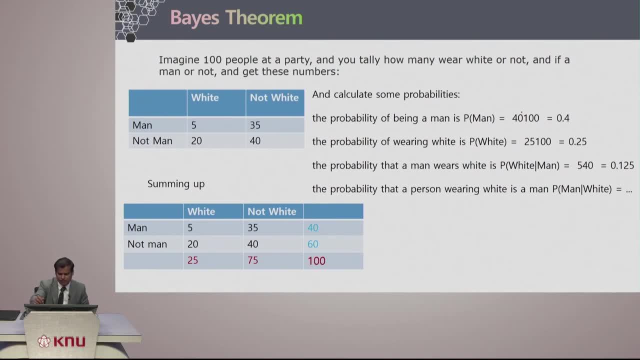 of being a man is probability of probability of man is 40 by 100, which is 0.4.. And probability of wearing white is 25 divide by hundred, which is 0.25.. And probability of man wears: 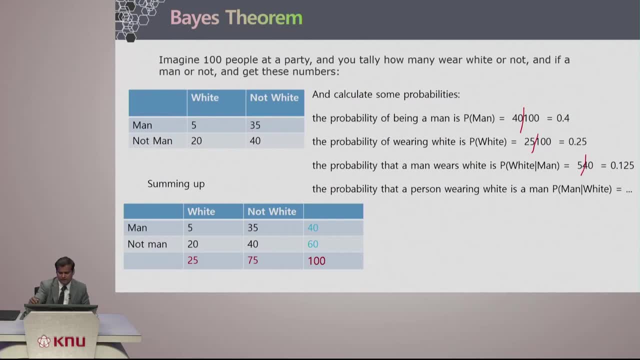 white is 5 divided by 40. That is 5 divided by 40,, which is 0.125.. So probability that a person wearing white is a man is probability of man, given he wears white. 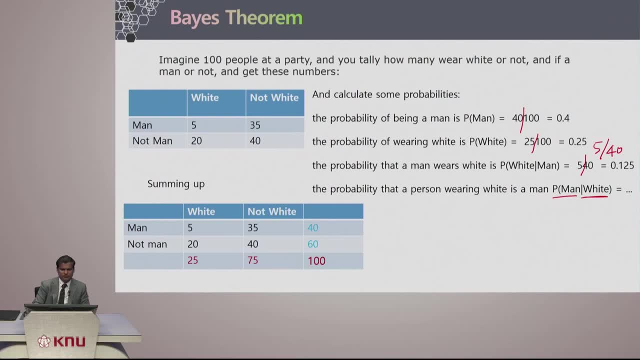 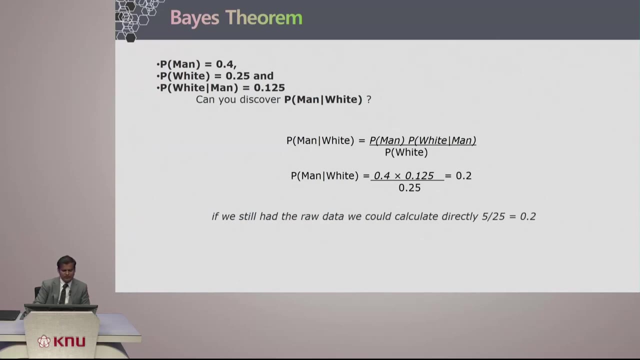 to check that out. Probability of person wearing white is a man, Probability that a person- the guest- who is wearing white is a man. So with this given information, can you discover the probability of a person who is man and wearing white. So with this thought, we can. 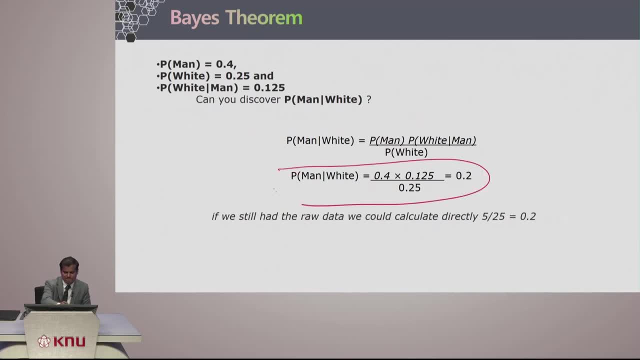 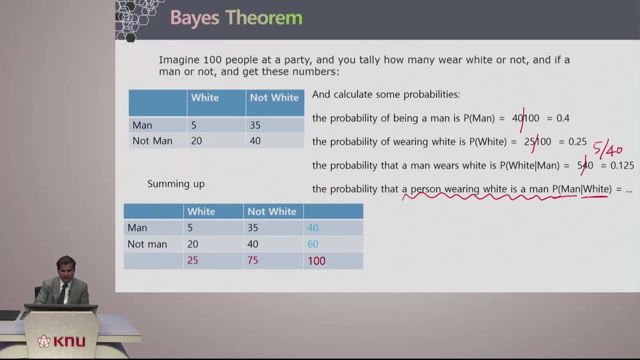 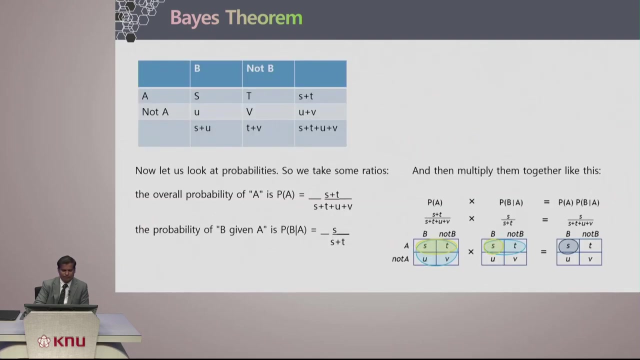 calculate using this formula here. In this case we have 0.25.. There is 0.2 here, So it is a raw data. We can also calculate directly. If you look at closely, you can also see that how this is being applied: 5 by 25.. Well, with this thought, we can calculate the probability. 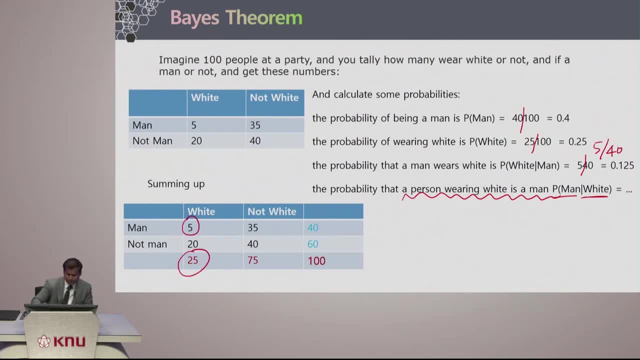 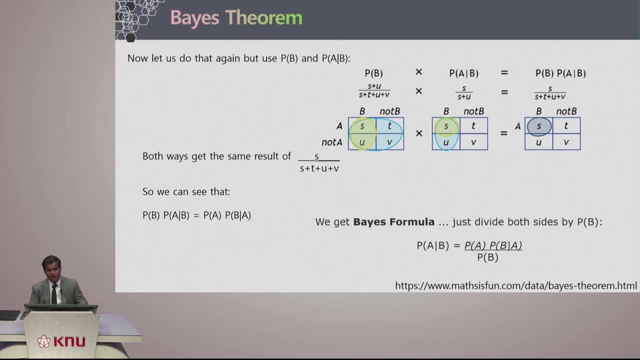 of a person wearing white. With this thought, let us move on to some common terms. Even without having applying these numbers, you can also see how you can use certain characters to understand what is there and what is not there. We talked about man and not man- white. 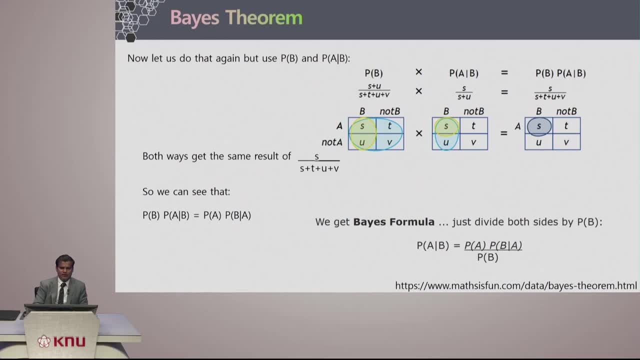 and not white. So based on that, you can see you can fill this similar structure with S T U V And you can see you can use the same formula here and apply the same principle for the given problem here. So for example, S plus U, divided by S plus T, plus U plus V, for all. 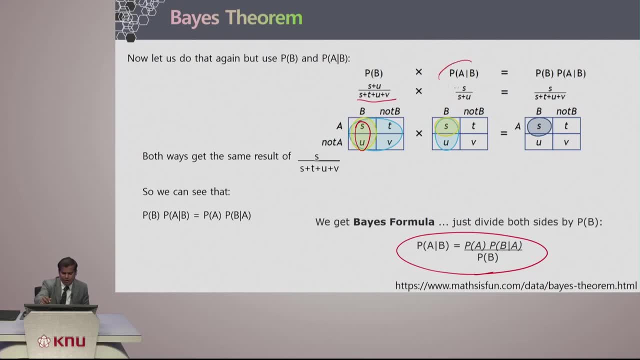 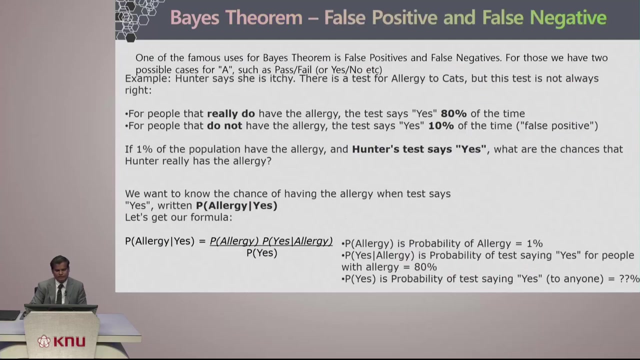 of probability of B And probability of A given B is S divided by S plus U. That is probability of A given B, Probability of B times probability of A given B. we have just S, So with this you can fill in the information like that, as we have just seen. 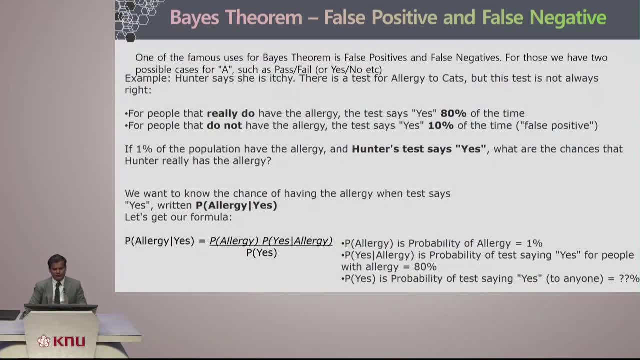 here There is more information on false, false-positive and false-negative. So this is another feature of the Bayes theorem, Not only the Bayes theorem, there are lot of other other areas in machine learning. we always want to consider this: false, positive and false. 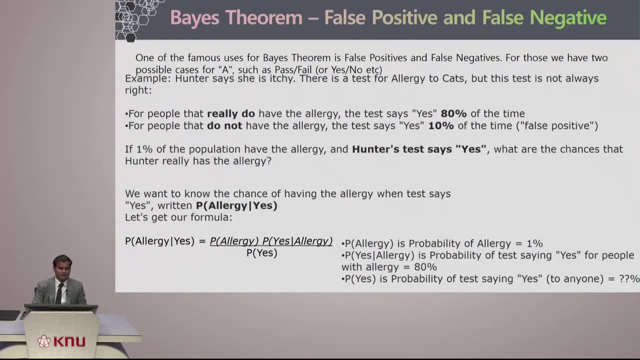 negative information because at times, it is of prime importance. You can consider this example here: Here, hunter says she is itchy. She says she is itchy and there is a test for allergy for cats, but this test is not always right, which means that they are not. 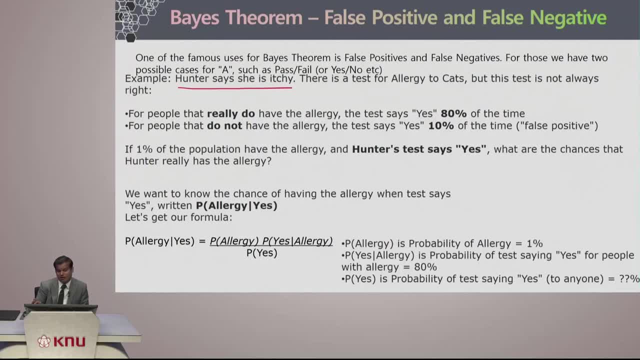 100 percent accurate. So the people really do have allergy. So when you take a test when a person really has an allergy, the test says 80 percentage of time it gives you correctly. But when you take a test when a person really has an allergy, the test says 80 percentage. 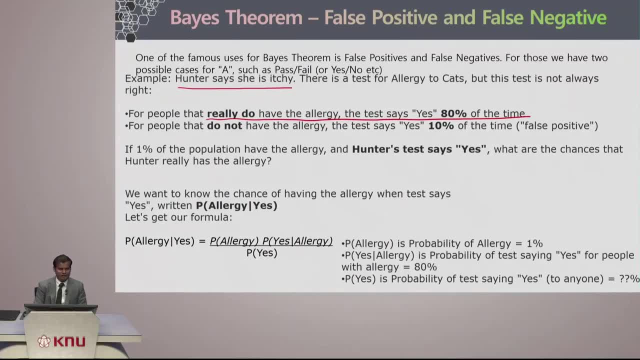 of time it gives you correctly. But for people who do not have allergy, the test says yes, they have allergy, 10 percentage of time, which means that is your false positive, Just like you go and test for influenza and even if you do not have influenza, you have been tested as influenza, something like that. 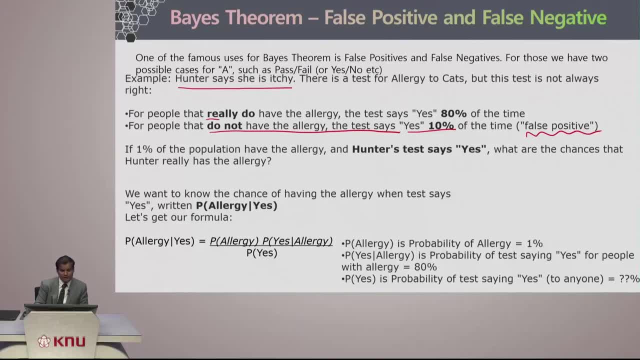 So if 1 percentage of the population have allergy and 100 tests says yes, what are the chances that hunter really has the allergy? So we know that chance of having allergies when test says yes is probability of allergy. given that the test says yes, the person has. 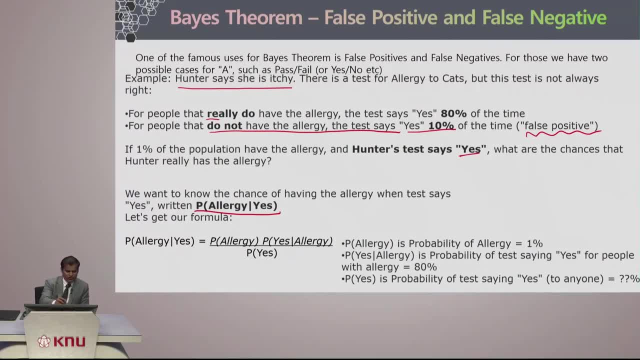 allergy, That can be written as probability of allergy, times probability of S, given that there is an allergy divided by probability of S. So when I say yes, which means that the test says positive, the person has allergy. So p of allergy is the probability of allergy. 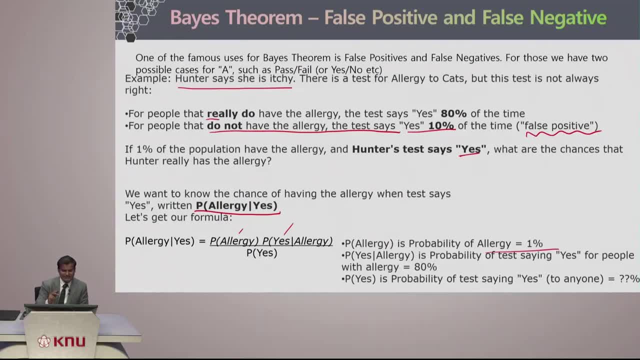 That is 1 percentage in the population, And probability of S- the test says yes and the person really has an allergy- is 80 percent. 80 percent it is accurate. you can say it gives the results correctly and probability of yes is a probability of test that says yes to. 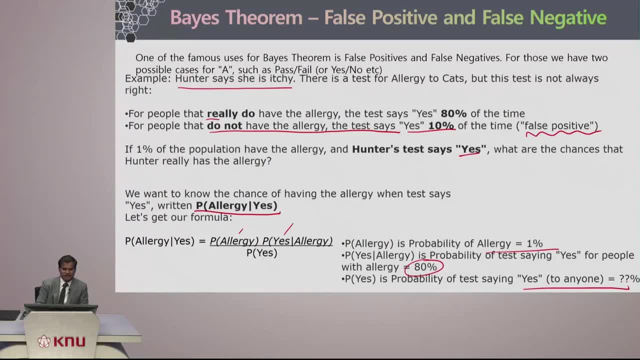 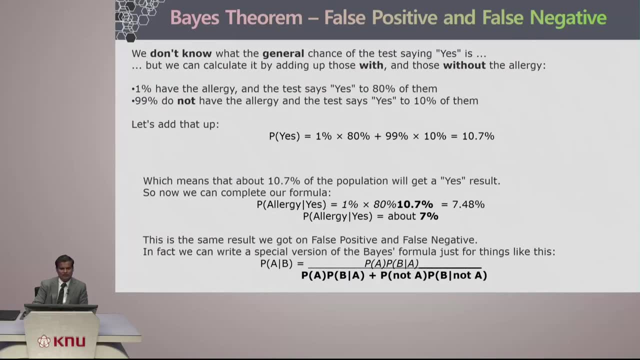 anyone. So we are not sure who they are like, whether they really has an allergy or not. Let us consider some information. We do not know what the general chance of test saying yes is, but we can calculate just by adding up those with and those without the allergy. 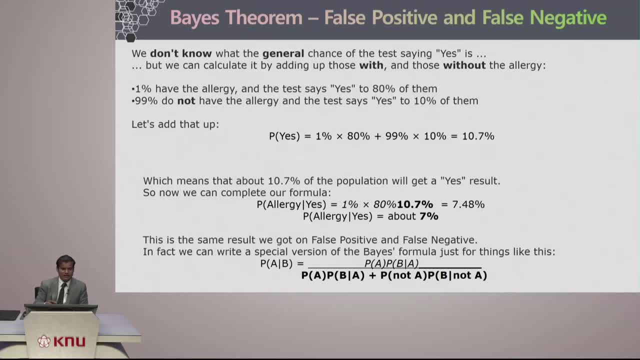 So we know that one percentage in the population has allergy and when an allergic person tested 80 percentage of them or given positive results like yes, as a result, 80 percentages and 99 percentage do not have allergy, but the test says yes to 10 percentage of them, which means 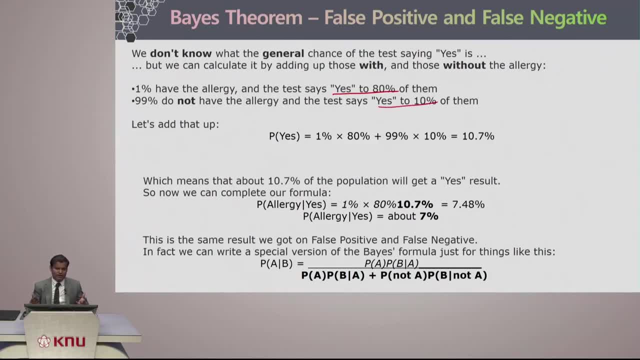 even if you do not have allergy, you can say yes to 10 percentage of them. which means, even if you do not have allergy, you can say yes to 10 percentage of them. which means you can calculate 1 times and 1 percentage times 80 percentage plus 99 times 100 percentage. 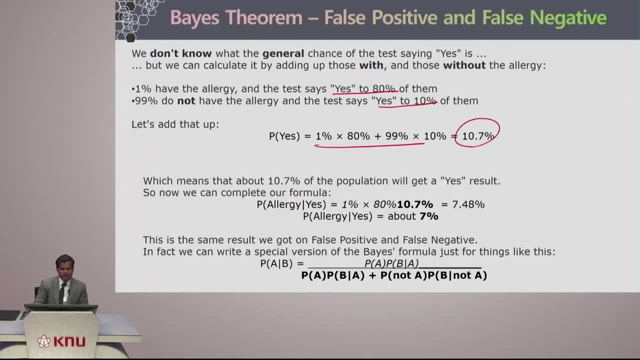 which is 10.7.. So with this, 10.7 of the population will get yes results. actually, Now, probability of a person gets higher by 10, because once you have 10 percentage of them- foretas, I had 10 percentage- 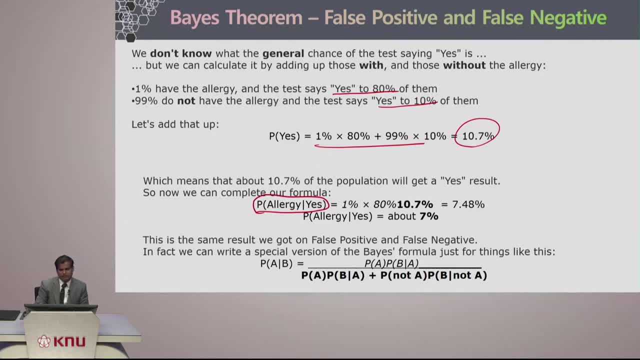 So twice person being allergic, given that the positive results. So 1 percent in the population, 80 times when you calculate it it gives us 7.48 percentage. So with this information we can move ahead and try to understand what is happening like probability of allergy. 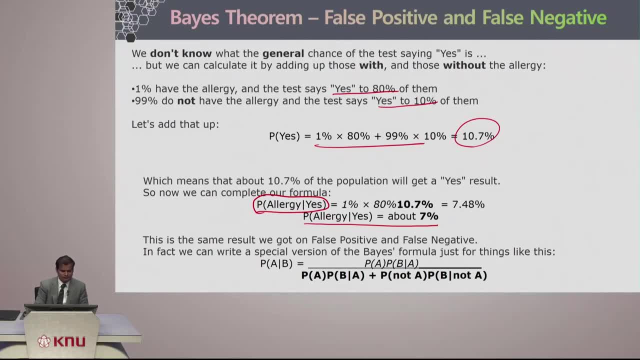 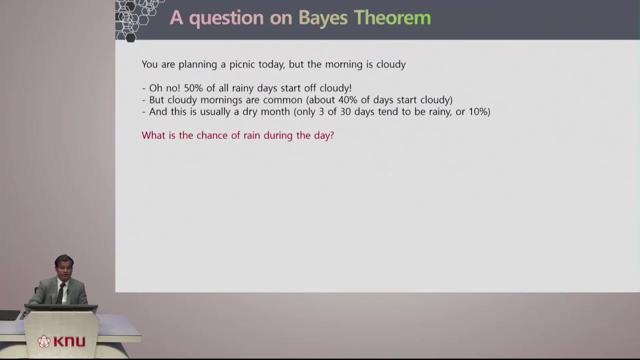 given yes is about 7 percentage. So this is same result as we got for false positive and false negative. So you can use the base formula again in this aspect to check the false positive and false negative. So, finally, we move on to this question. I leave these questions for you. You can try. 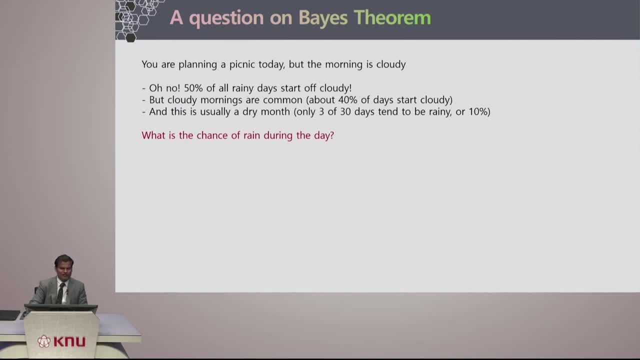 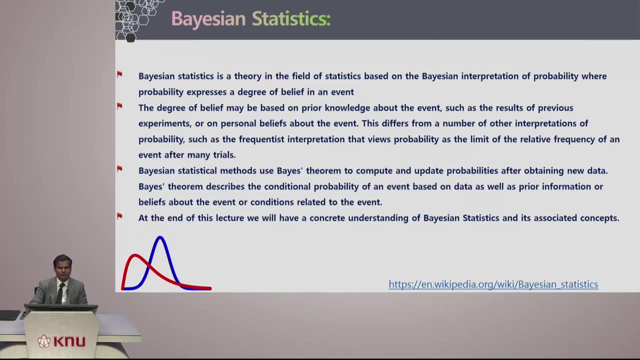 to solve this question by yourself. It is a simple question related to Bayes' theorem. You have to find the chance of rain during the day. Basically, the Bayesian statistics is a theory in the field of statistics based on certain Bayesian interpretation of probability, where the probability expresses a degree of belief. 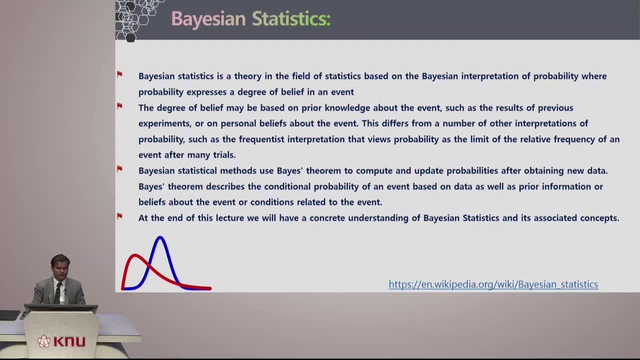 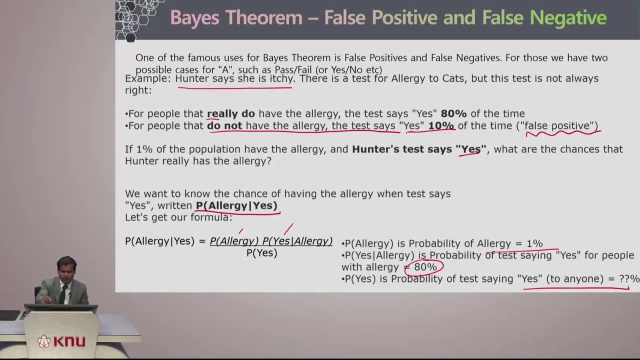 in an event. In the previous example we saw that the degree of belief is that 1 percentage of the population has the allergy. but we believe that 80 percentage of the test shows accurately positive. but still there is a chance, like we had 10 percentage, we get the false positive. 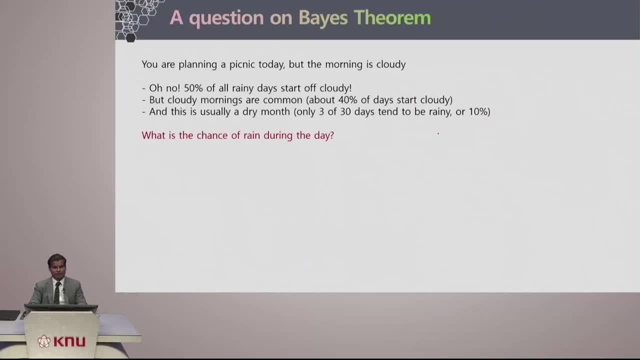 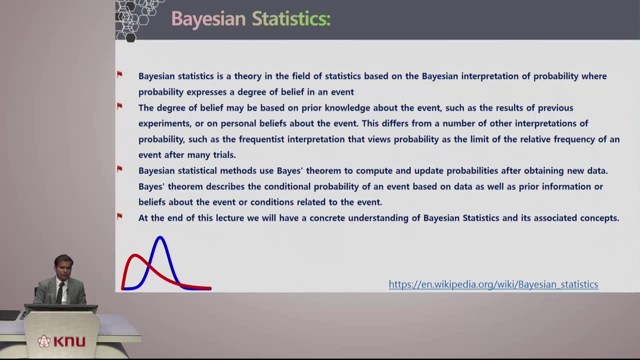 in this example. So, based on certain beliefs, we can get the false positive. So, based on certain belief of an event, we proceed to find the actual probability by means of certain interpretations and experiments. So such interpretations can also be interpreted using frequentist interpretation. In other 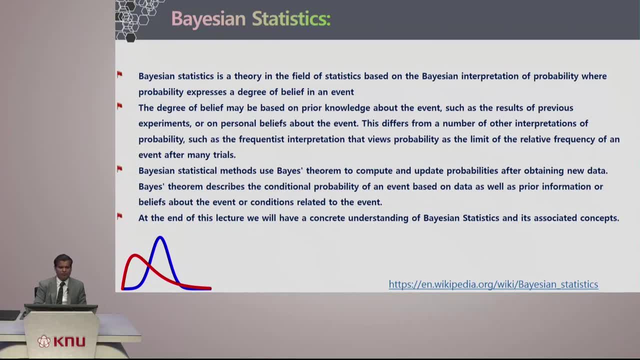 words, how frequently things are going to be happening and how we can interpret and infer things from those conditions or conditional probabilities or events. 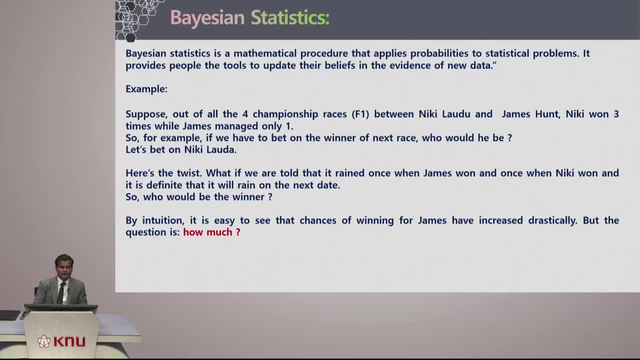 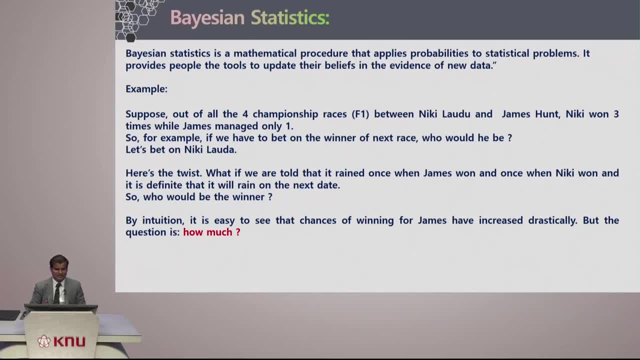 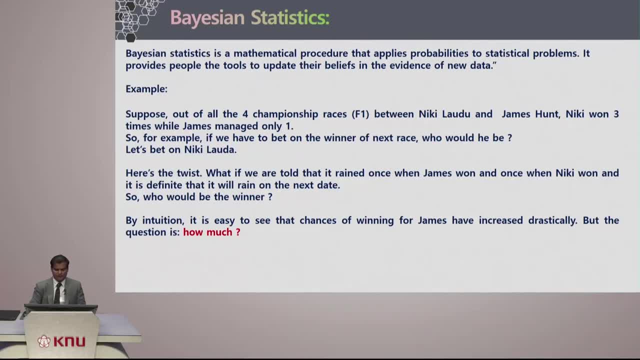 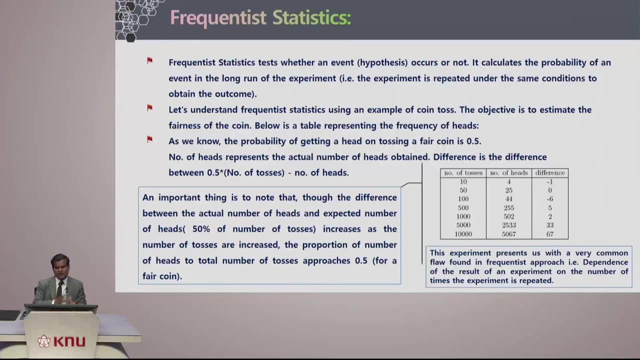